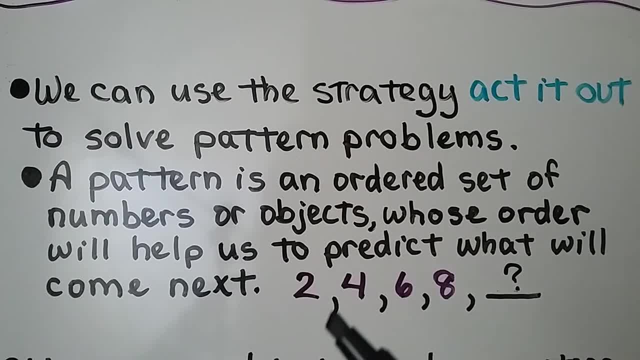 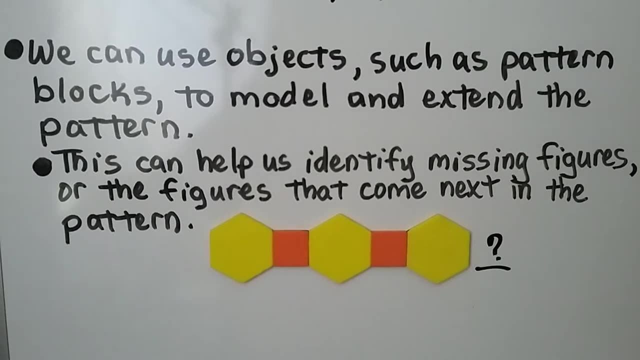 If you looked at what was happening with the numbers, there is skip counting by 2.. The next number would be 10.. The order helped us predict what will come next. We can use objects such as pattern blocks to model and extend the pattern. This can help us identify missing figures or the 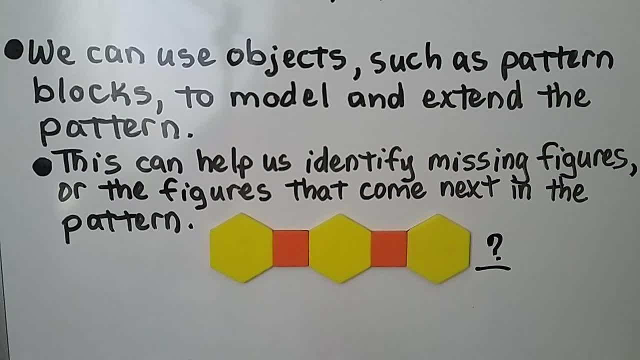 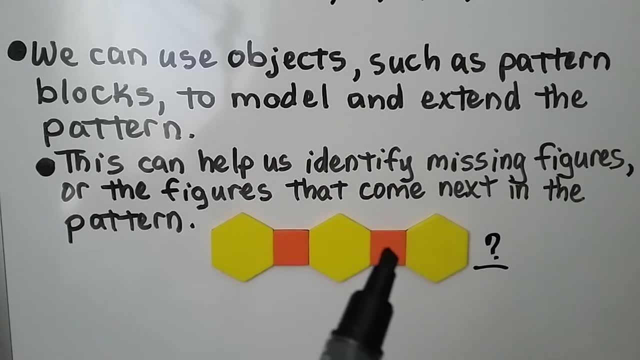 figures that come next In the pattern we have this: a yellow hexagon and an orange square. a yellow hexagon, an orange square, a yellow hexagon. Can you figure out what comes next? If you said orange square, you're right. 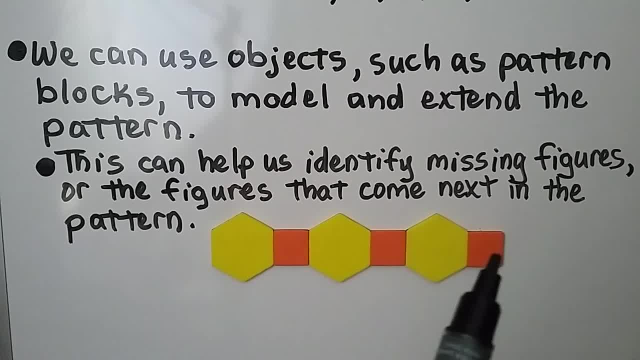 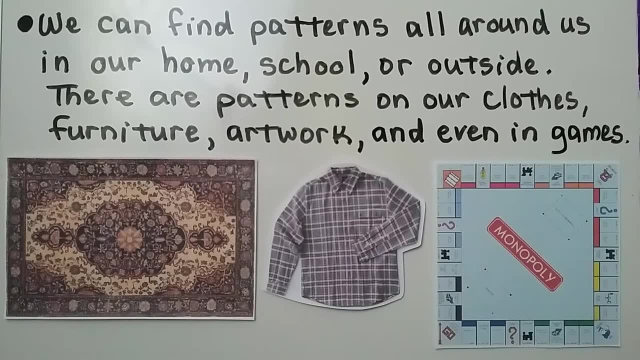 The order of these pattern blocks helped us predict what would come next. We can find patterns all around us, in our home, school or outside. There are patterns in our clothes, furniture, artwork, even in games. Look at this rug. Do you see the pattern? We can even see it has line symmetry. 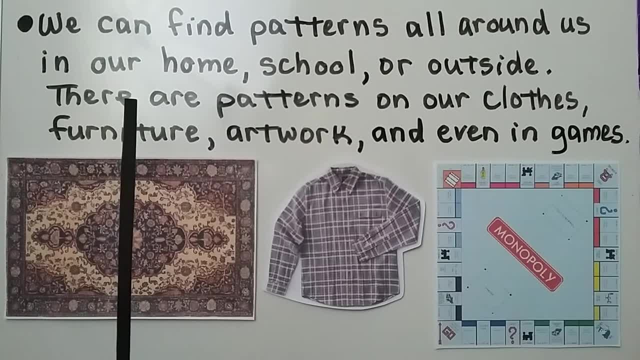 If we put a line like this, we see the two sides match. It even has horizontal line symmetry, doesn't it? And the pattern of the shirt is plaid: The stripes are white, and then a dark brown and then a white. 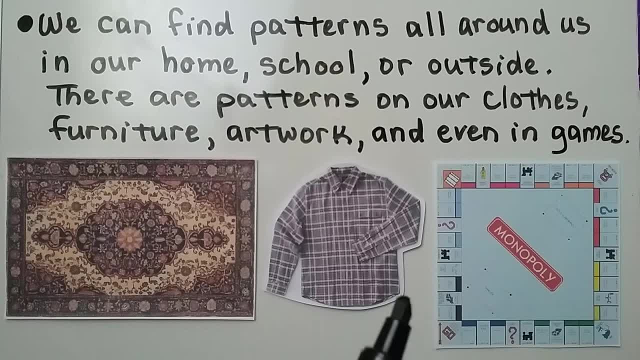 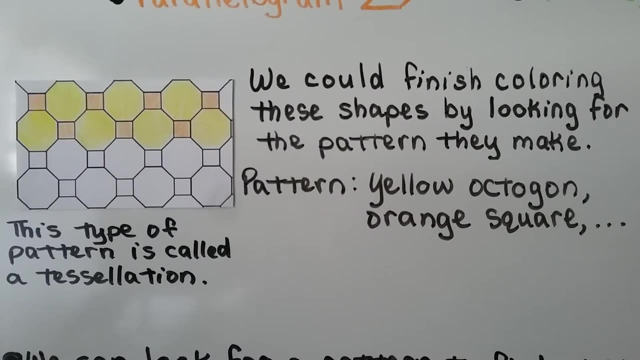 There's a pattern there. Even in the game we can see there's a railroad in the middle, a railroad in the middle, a railroad in the middle and a railroad in the middle. There's a pattern to that game. We could finish coloring these shapes by looking for the pattern they make. 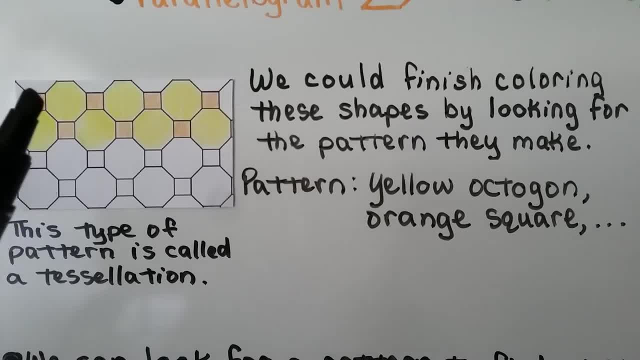 The pattern is a yellow octagon and an orange square, and they're taking turns, aren't they? This type of pattern is called a tessellation, But by looking at what's happening with the yellow octagons and orange squares, we could finish coloring it. 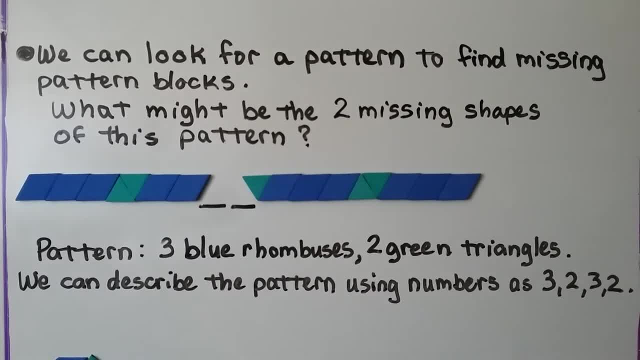 We can look for a pattern to find missing pattern blocks. What might be the two missing shapes of this pattern? We see three blue rhombuses, then two green triangles, And then there's only two blue rhombuses and one triangle, but then there's three again, and two again and three again. 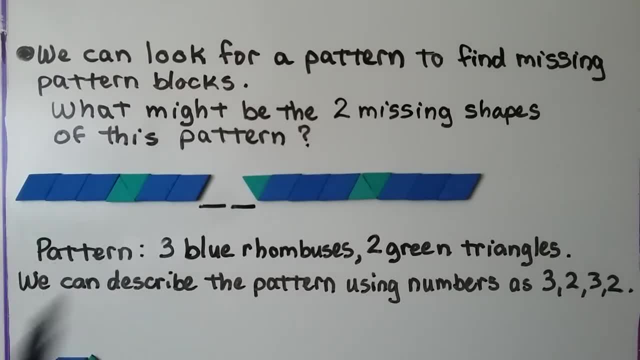 So the pattern must be three blue rhombuses. There must be two blue rhombuses and two green triangles. There must be a blue rhombus and a green triangle missing. We found the pattern and we can complete the missing pieces. 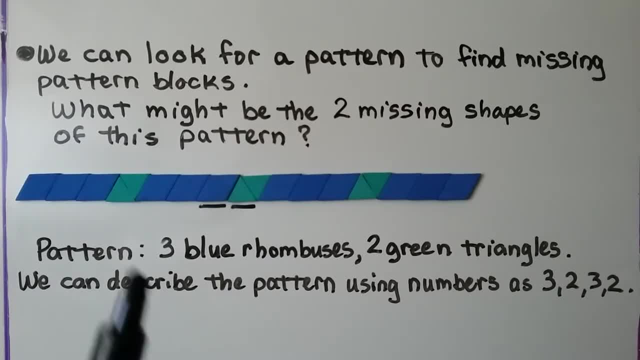 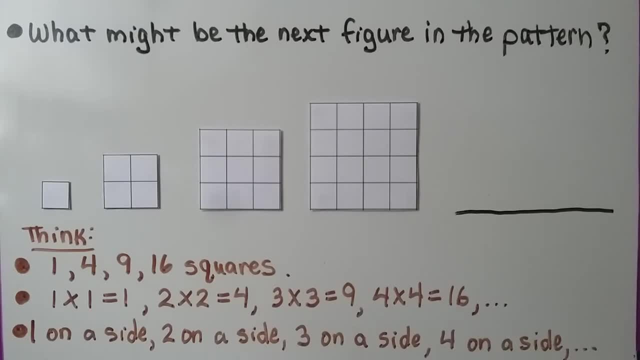 So what might be the next figure in the pattern? I see there's 1 square, 4 squares, 9 squares, then 16 squares. What would go here? We can think: 1 times 1 is 1.. 2 times 2 is 4.. 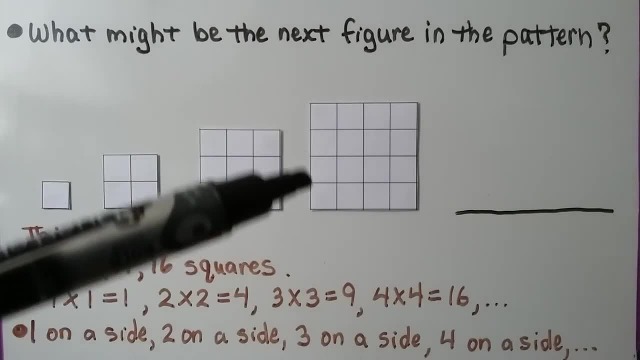 3 times 3 is 9.. 4 times 4 is 16.. This one must be. 5 times 5 is 25.. There's 1 on this side. there's 2 on this side. 3 on this side, 4 on this side. 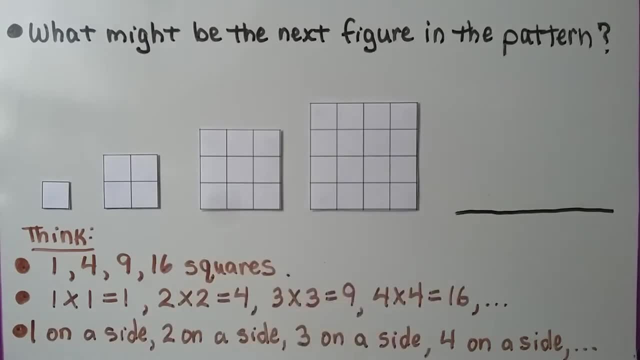 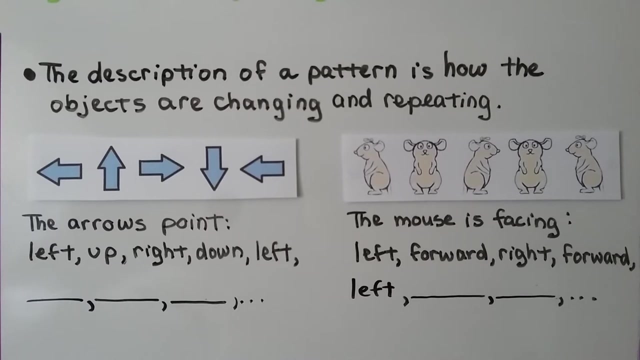 It must have 5 on the side and 5 going across the top, And we would know the very next one after this one would be: a 6 times 6 equals 36.. 36 squares: The description of a pattern- is how the objects are changing and repeating. 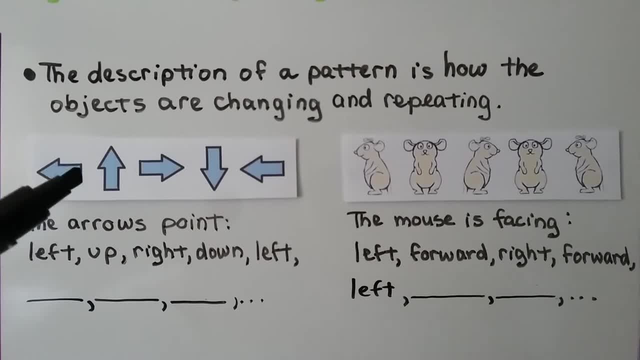 We have some arrows here, And the arrows are pointing left up, right down, then left again. Do you know what would be the next direction for this space? Well, after left came up, so it must be up- What might the next direction be? 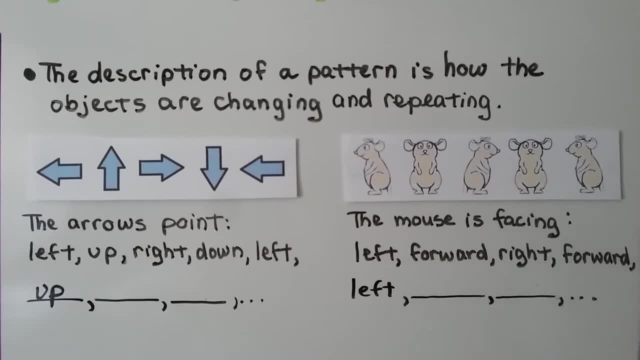 Well, after up it pointed to the right, And after it pointed to the right, it pointed down. So that must be down, And the pattern would keep repeating. Now, what would happen if we only had one or two arrows? What if we only had these two arrows, the left and the up? 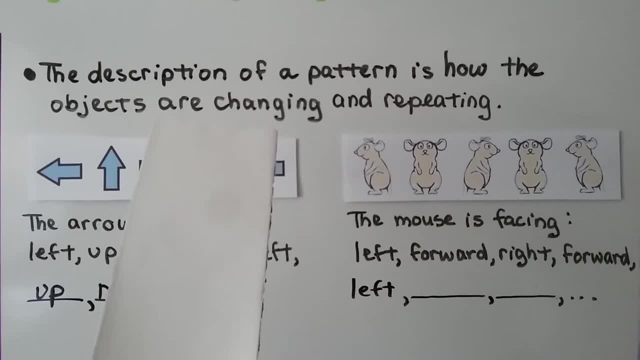 Would we know what the next direction in the pattern would be? Well, that would be really hard. We don't have enough objects to know what the pattern is. We've only got two, And even if we had three, we wouldn't know if we have the pattern correct. 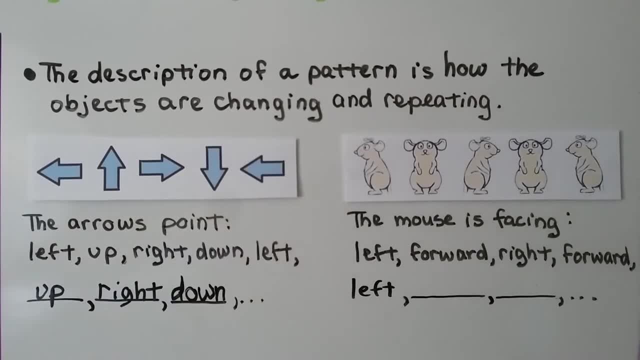 So we need several objects to know what a pattern is These little mice? this little mouse is facing to the left, This one's facing forward, And this one's facing to the right, And this one's facing forward. Then he's facing to the left again. 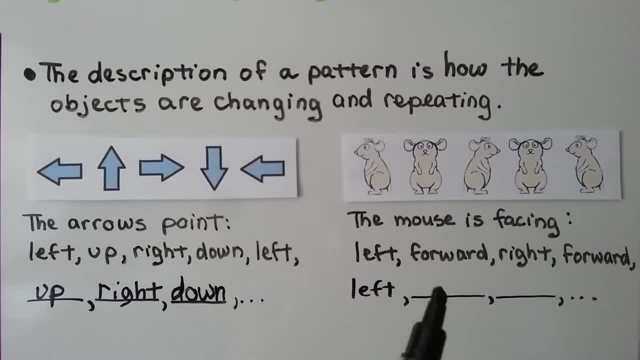 So what direction would the mouse be facing for the next space? He went left forward, right forward, left. If you said forward, you're right, You're correct. And what would go in this space? What direction would he be facing? 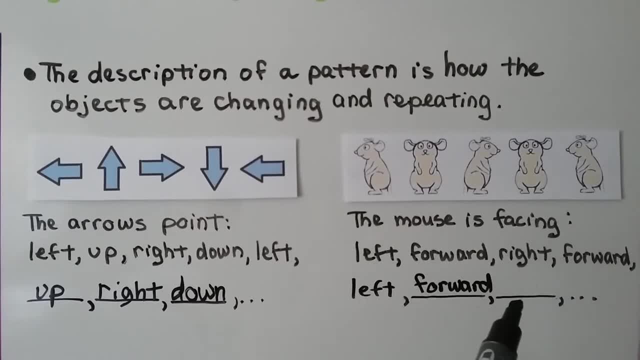 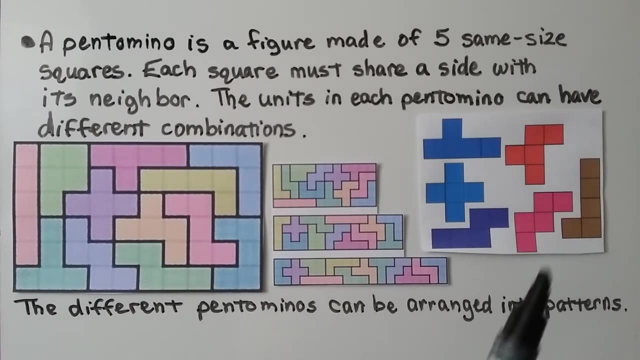 We've got left forward, It would be facing in the right direction, And we could keep repeating this pattern. The pentomino is a figure made of five same-size squares, And each square must share a side with its neighbor, And the units in the pentomino can have different combinations. 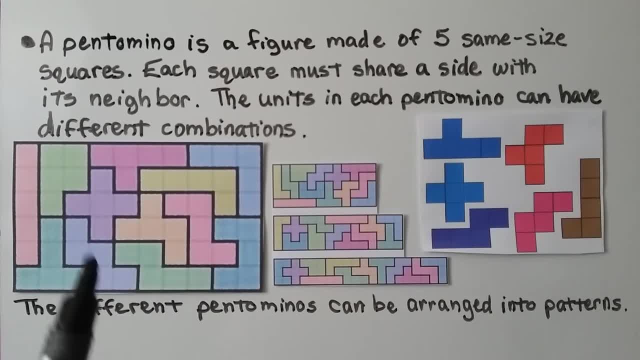 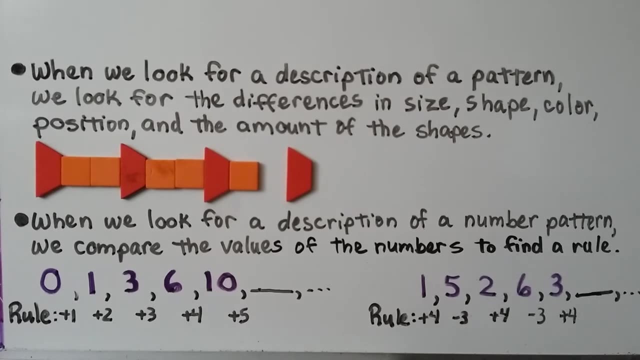 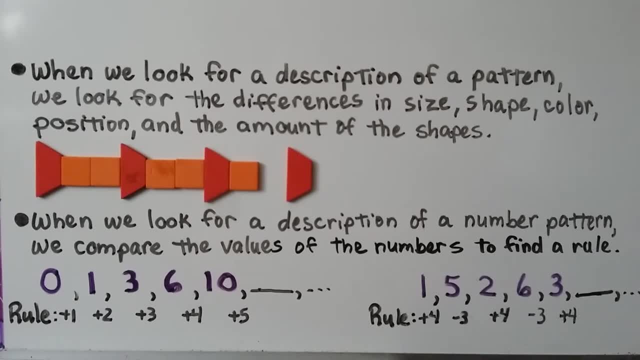 Can you tell which shape is missing from this pattern? We have a trapezoid, then two squares. a trapezoid, two squares, a trapezoid. Well, there should be a square, there, shouldn't there. 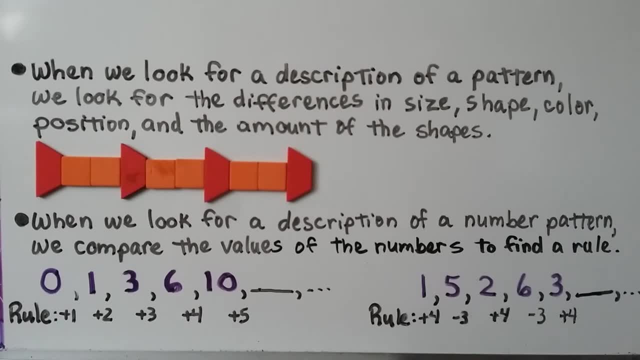 When we look for a description of a number pattern, we compare the values of the numbers to find a rule. The numbers go 0, 1,, 3,, 6,, 10.. And we ask ourselves: what's the difference between this number and this number? 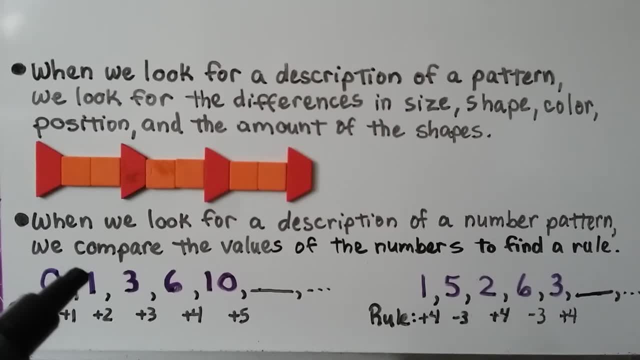 Well, 0 plus 1 is equal to 1.. And what's the difference between this one and this one? Well, 1 plus 2 is equal to 3.. And the difference between the 3 and the 6, 3 plus 3 is 6,. 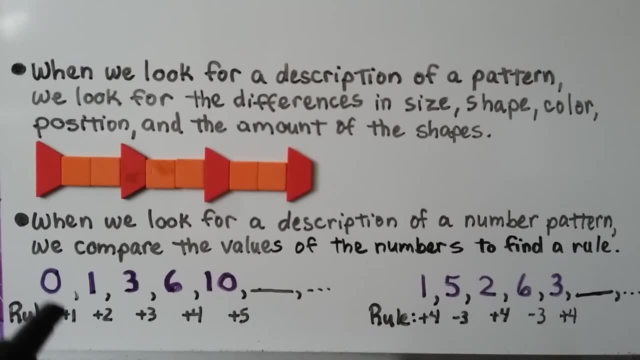 we can start to see the pattern that the numbers are going from 0 plus 1 plus 2 plus 3, and then 6 plus 4 is 10.. So do you know what would go in that space? We would have 10 plus 5.. 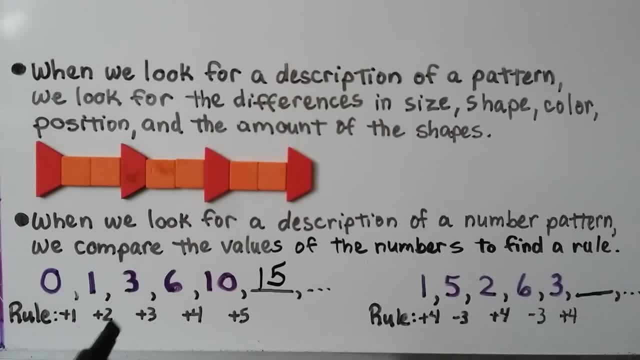 So the rule for this number pattern is plus 1 plus 2, plus 3, plus 4 plus 5, and we could keep going. We could keep adding more numbers. For this one, our numbers are 1, 5,, 2,, 6,, 3, and then we have a missing one. 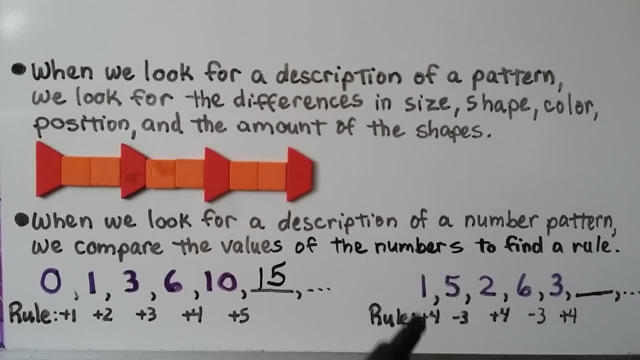 We ask ourselves the difference between the 1 and the 5.. Well, 1 plus 4 is 5.. Then we have a 2.. And the difference between the 5 and the 2, we took away 3. And if we look at the numbers we can see the rule is plus 4, minus 3.. 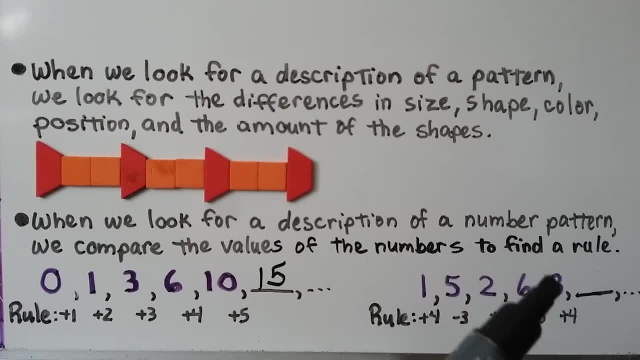 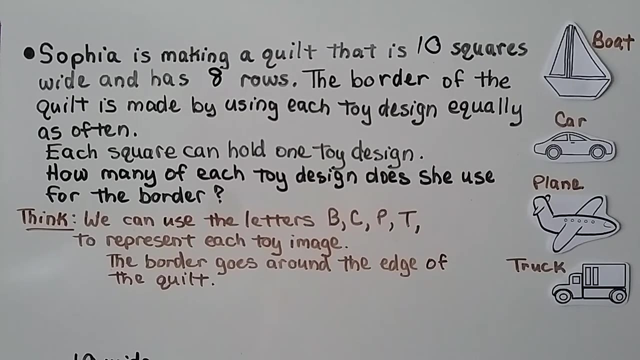 Plus 4 minus 3.. Plus 4, we'd have 3 plus 4.. Do you know what would go in that space If you said 7,? you're correct. Sophia is making a quilt that is 10 squares wide and has 8 rows. 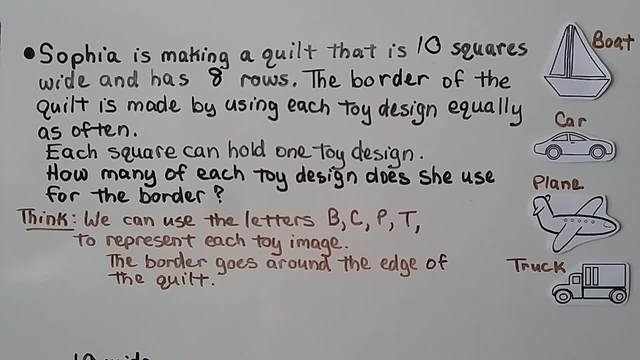 And the border of the quilt is made by using each toy design equally. as often That means she's going to use the same amount of toy designs. Each square can hold one toy design, So how many of each toy design does she use for the border? 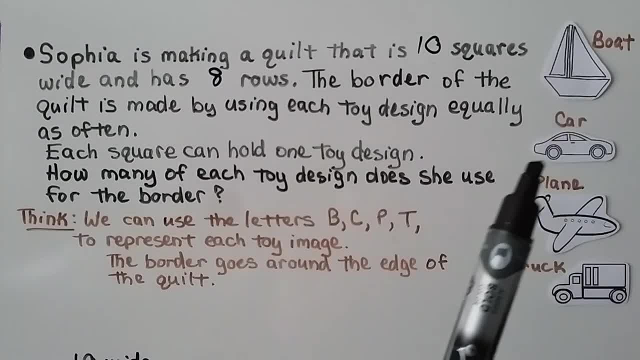 We think We can use the letters B for boat, C for car, P for plane and T for truck to represent each toy image. And the border goes around the edge of the quilt. The border would be this little space going around the edge of the quilt. 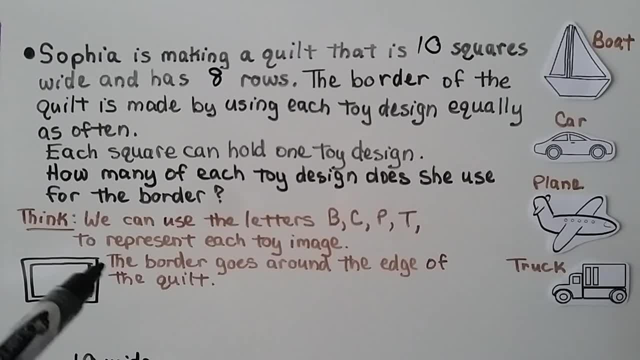 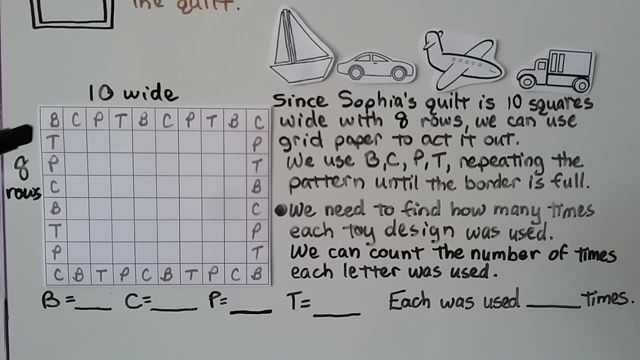 And she wants to put squares of the toy designs in them. It's 10 squares wide and has 8 rows. Since Sophia's quilt is 10 squares wide with 8 rows, we can use grid paper that has 10 squares wide and 8 rows. 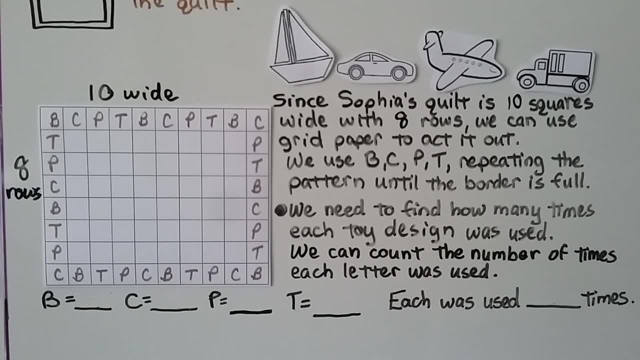 And we can use the BCPT repeating the pattern until the border is full. We can start up here in this corner and put BCPT and repeat it, BCPT, BCPT, going all the way around repeating the pattern. We need to find how many times each toy design was used. 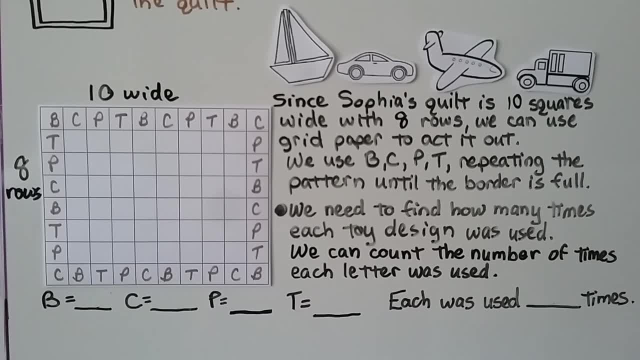 We can count the number of times each letter was used. We count how many B's there are: 1,, 2,, 3,, 4,, 5,, 6,, 7,, 8.. That means she used the toy boat figure 8 times. 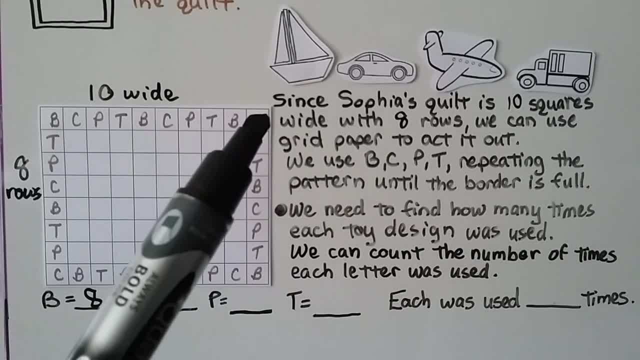 We can count the C for car: 1,, 2,, 3,, 4,, 5,, 6,, 7, 8.. 1,, 2,, 3,, 4,, 5,, 6,, 7,, 8.. 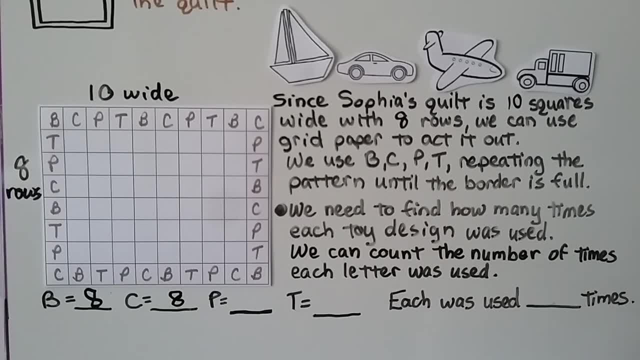 Then we can count the P's for plane and the T's for train. We could also count how many times the entire pattern is repeating. We have 1, 2, 3, 4, 5,, 6,, 7,, 8.. 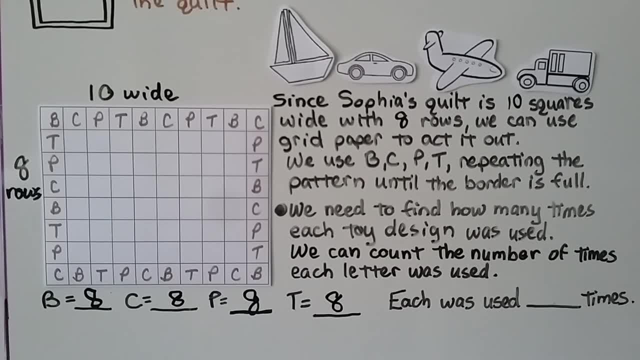 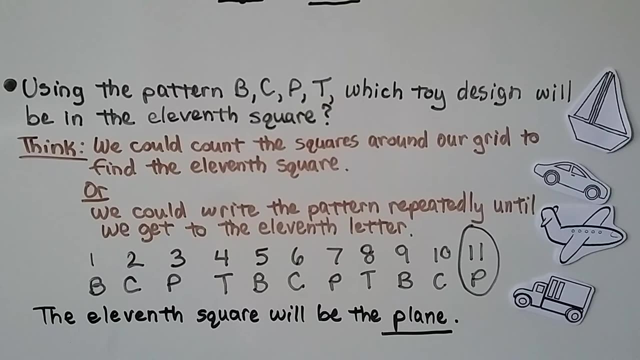 They're all repeating 8 times. That means each toy image was used 8 times And the pattern repeated all the way around the border, Using the pattern BCPT for boat, car, plane, train. which toy design will be in the 11th square? 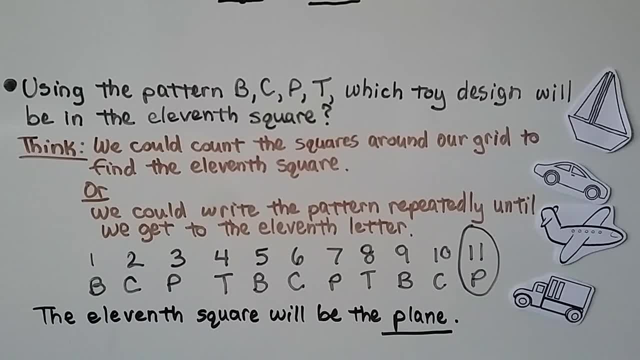 So we think we could count the squares around our grid to find the 11th square, and that would be the 11th toy. or we could write the pattern repeatedly: BCPT, BCPT, until we get to the 11th letter, BCP. 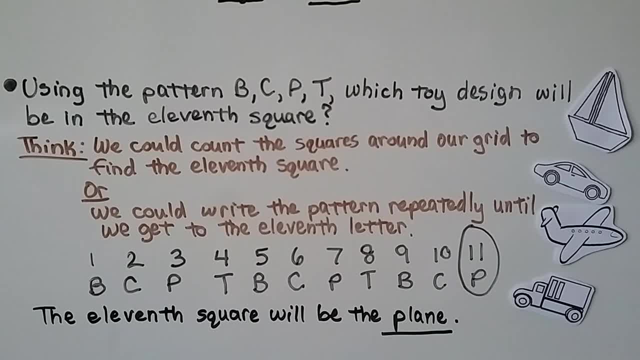 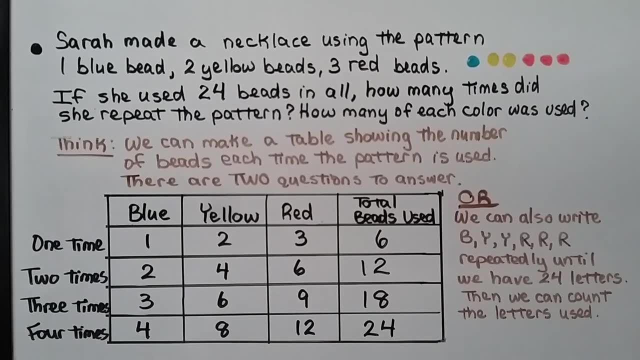 And the 11th square would be the plane. Sarah made a necklace using the pattern: 1 blue bead, 2 yellow beads, 3 red beads. If she used 24 beads in all, how many times did she repeat the pattern? 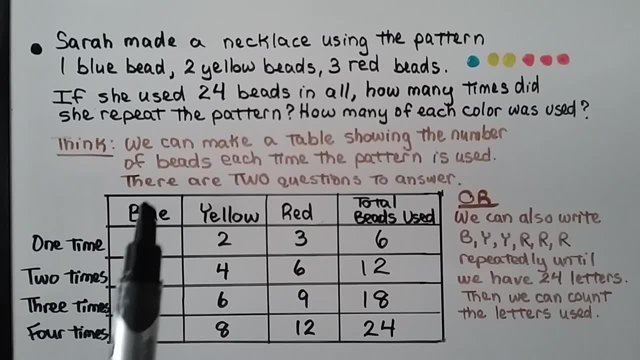 How many of each color was used. So be careful. there are 2 questions to answer: How many times did she repeat the pattern and how many of each color was used? And we can make a table showing the number of beads each time the pattern is used. 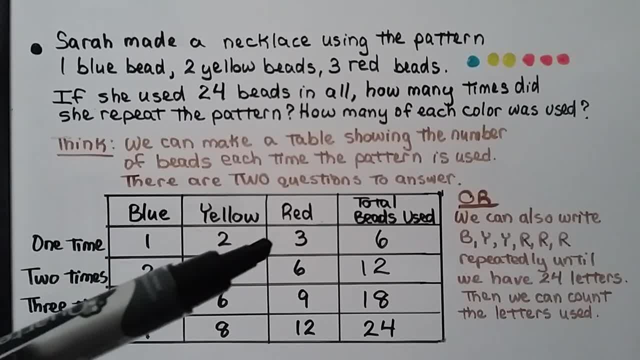 There's 1 blue bead, 2 yellow beads and 3 red beads. if she uses it 1 time, That's a total of 6 beads used. If she does it 2 times, then we're going to have 2 times 1 blue bead. 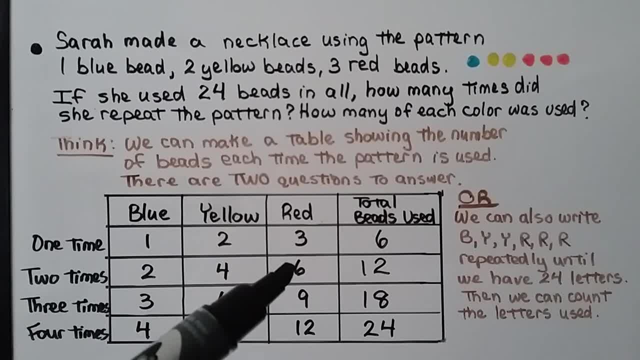 2 times 2 yellow beads and 2 times 3 red beads. That'll be a total of 12 beads used. We can repeat on our table 3 times. would be 3 blue, 6 yellow, 9 red, with a total of 18,. 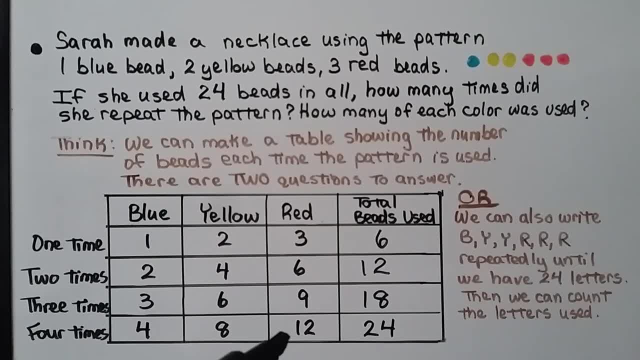 and then 4 times would be 4 blue, 8 yellow, 12 red and 24 beads, And that's how many she used in all. So we know she used 4 blue, 8 yellow and 12 red. 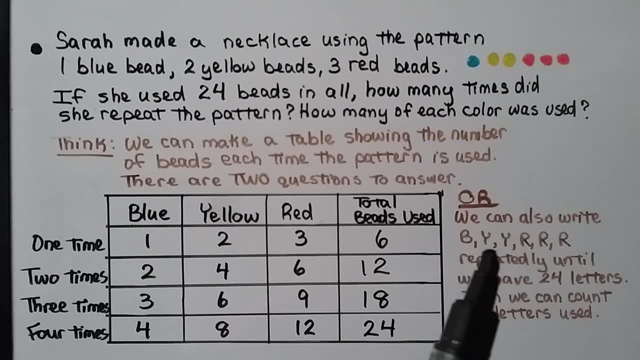 Now we also could have written B for blue, Y for yellow and R for red, And because there's 1 blue, we do 1 B, 2 Ys for 2 yellows and 3 Rs for 3 reds. 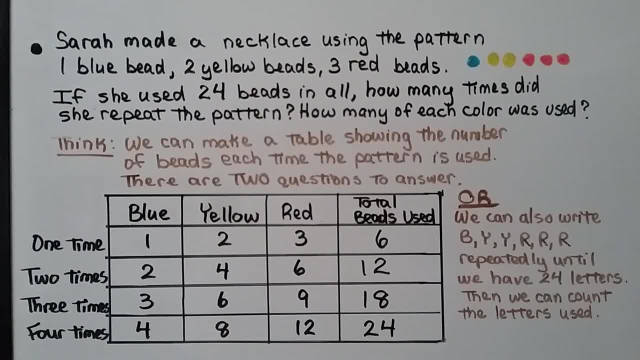 and repeat it until we have 24 letters and then count the letters used. That way we'll get the same answer. We need to remember there's usually more than one way to solve a problem. Some ways are easier than others. In our next lesson we're going to be in Chapter 11. 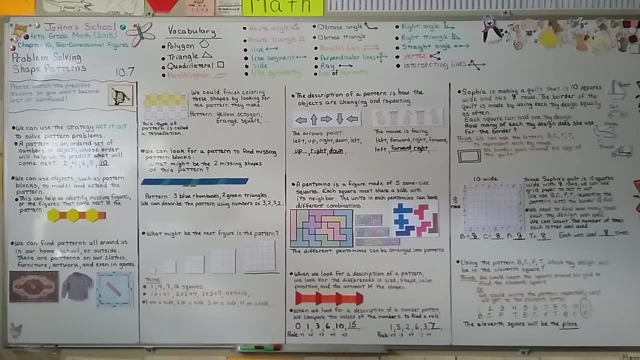 and learn about angles and how to measure angles. I hope you're having a great day and I am really proud of you for watching these math videos. I know I say it a lot, but I really am, And I'll see you next time. Bye.